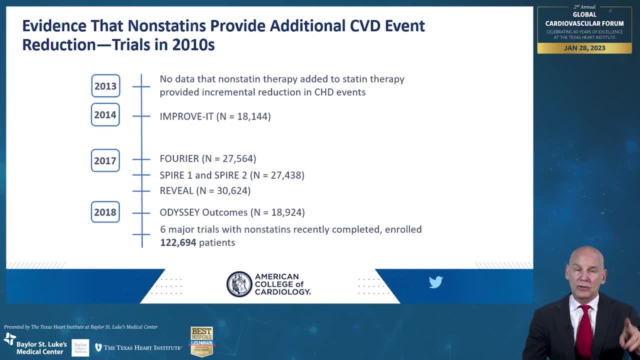 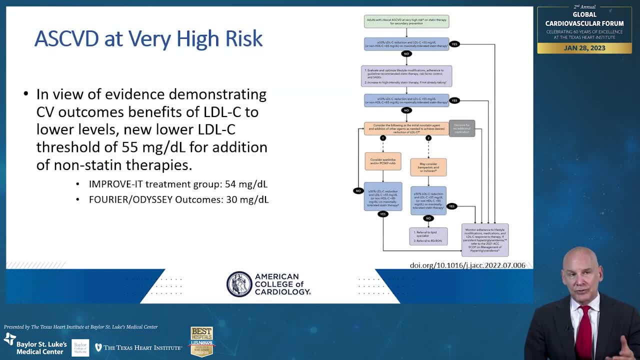 showing the benefit of adding non-statin therapies on top of statins to get further LDL reductions. All right. well, there's a lot of interest obviously in cardiology, in a patient with atherosclerotic cardiovascular disease who's at very high risk, and that's over half of your. 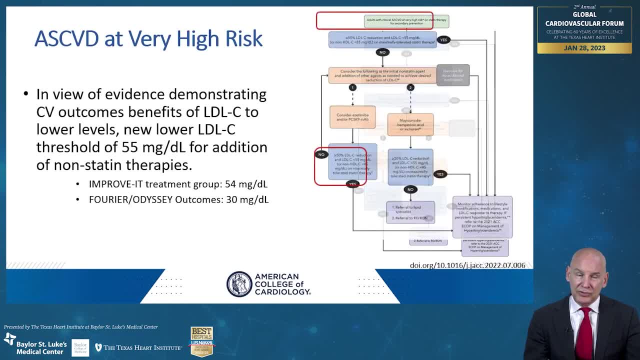 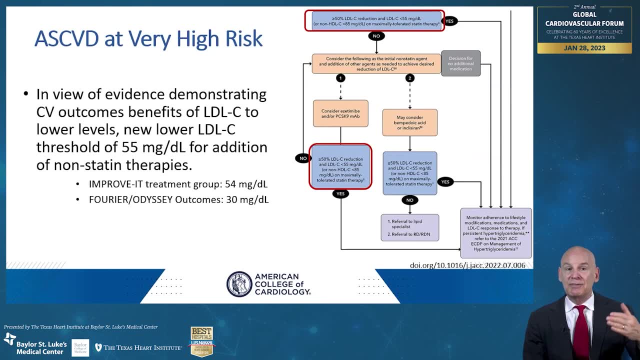 patients, And something new in these guidelines was that it's lowering now this concept of a threshold. If you've treated somebody with a statin, if the LDL is over 55, used to be 70, over 55, consider adding a non-statin therapy, And that was based upon the data from improvement. 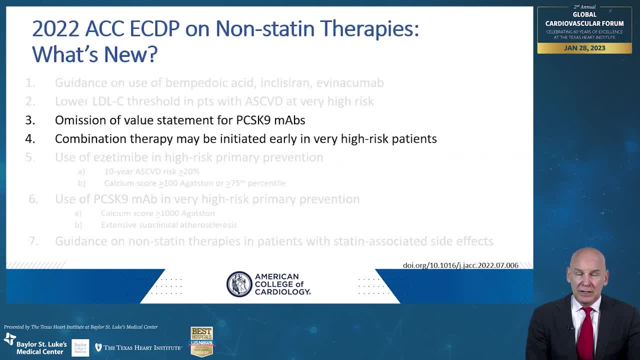 Fourier and Odyssey outcomes trials. Now they took out the value statement for the PCSK monoclonal antibodies because the price dropped considerably, went from $10,000 to $6,000 a year. That's a list price, That's not the actual price And there's more of a focus on 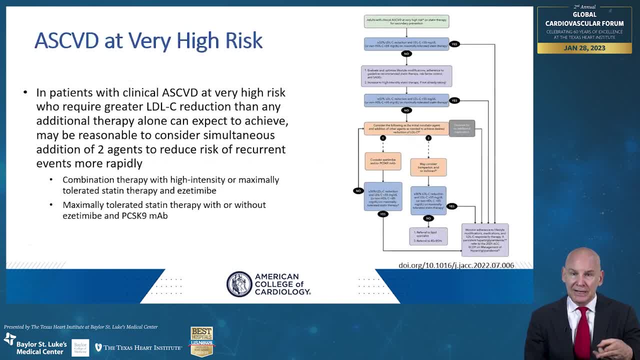 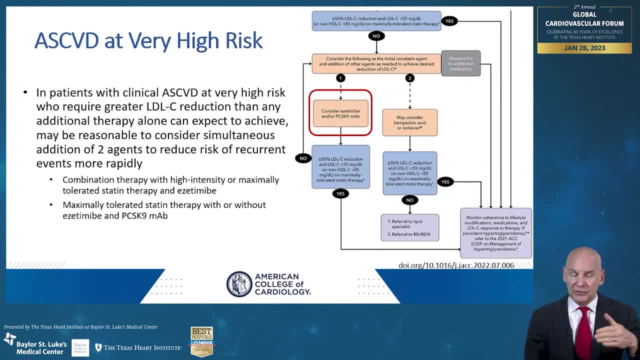 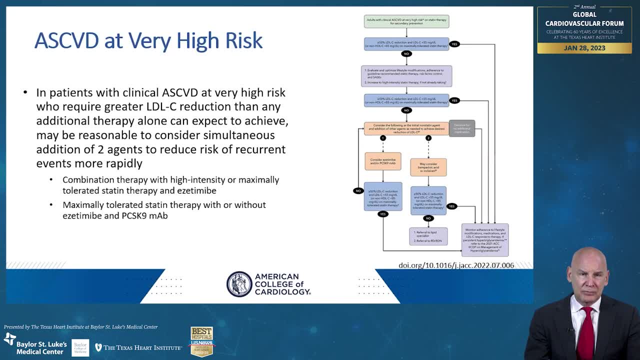 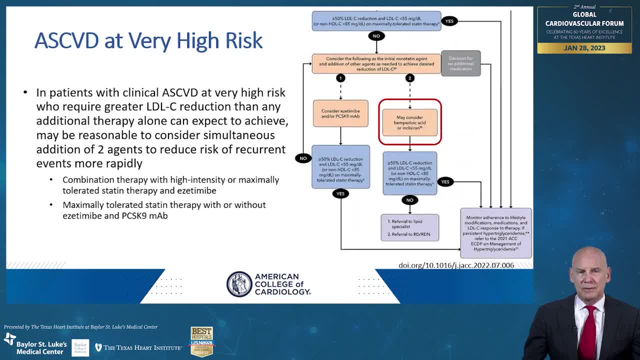 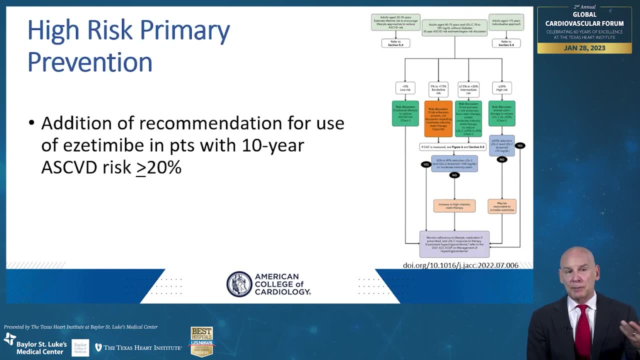 up is the focus in terms of getting there faster. So combination therapy, as we know, is going to be highly effective, And there's also the role of using some of our newer agents in these very high-risk patients to get them to target. What about high-risk primary prevention? Well, 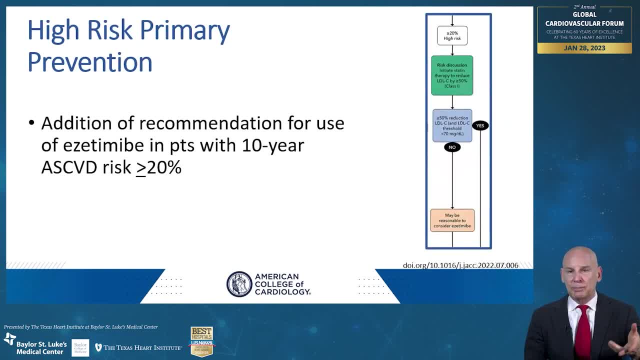 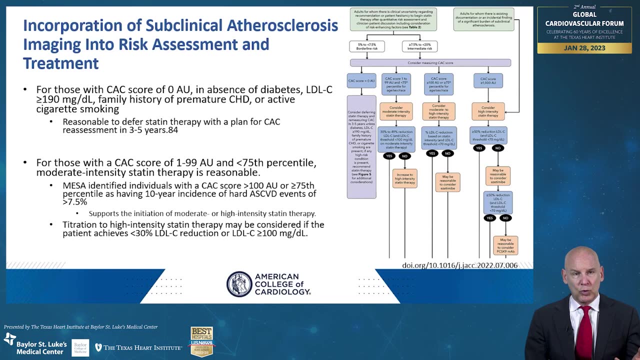 others. if people have a risk over 20%, consider adding ezetimibe there if you're trying to get LDLs down further. We know that combination therapy can be more effective than monotherapy. It's not used very much. And what about calcium scoring? That's become a very popular tool. We. 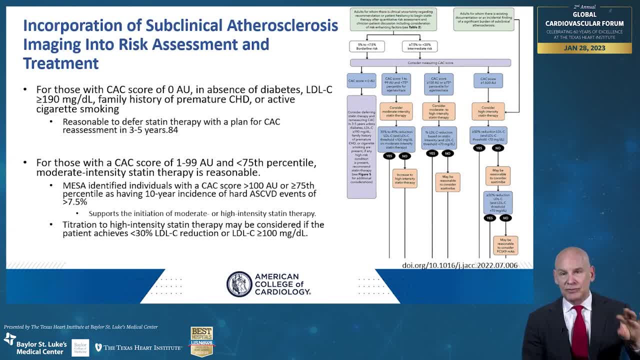 know it is very powerful for risk assessment. If you get a zero, you might defer statin therapy. If someone has calcium, well then you don't want to have at least moderate intensity statin therapy, But if it's over 100, that's someone that you might consider high-intensity statin. 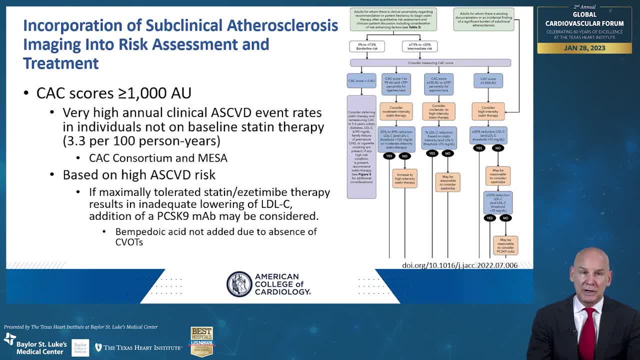 therapy, or also consider adding ezetimibe in those patients. What about if it's a very high score, like over 1,000?? Well, in this case, your risk is really: that person has extensive subclinical atherosclerosis, They've got lots of coronary disease, And so this ends up being 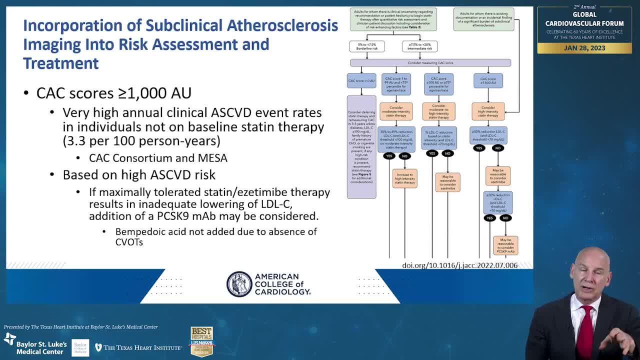 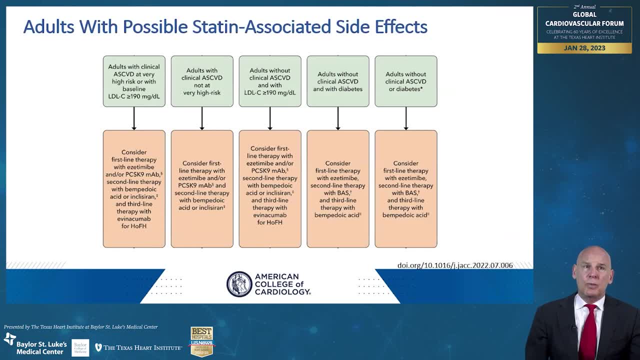 consideration of like using our very high-risk patients adding a PCSK9 inhibitor. All right, Now we all see people in our practice who really have a hard time with statins. Now it's very important if you look at secondary causes. Do they have a low thyroid, Do they? 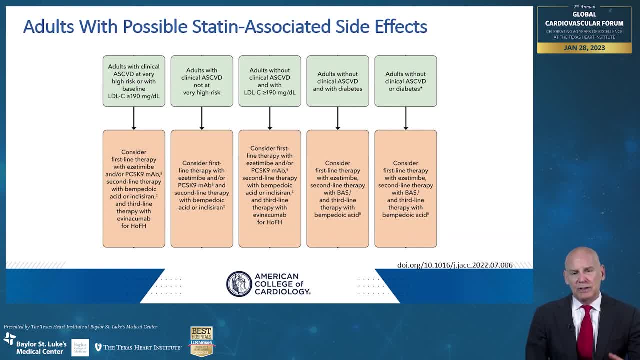 have some other issues that are going on in terms of myopathies. that might be a muscular disorder. It's important to try a different statin. You want to try lower doses. However, if you've marched through that and patients and I see people refer to me and they've referred to me and they've 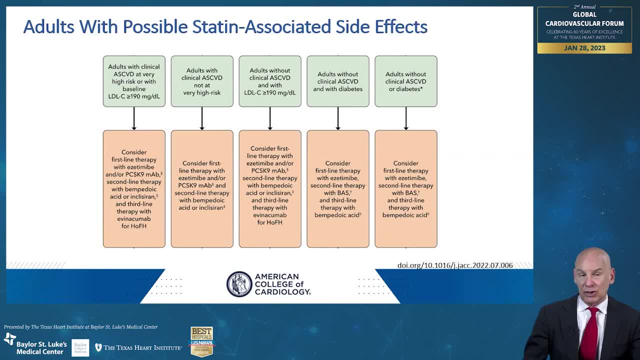 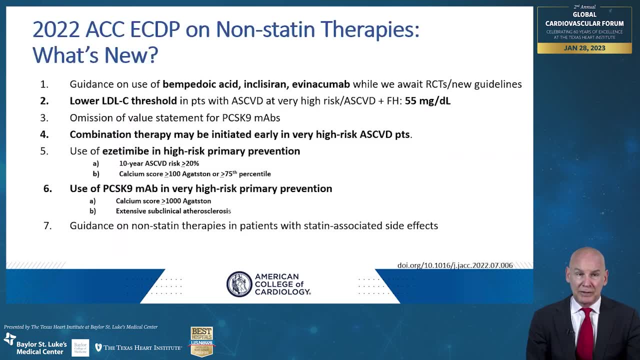 tried four different statins. They've also tried a low dose, the lowest possible dose of a statin. I will try every other day statin, sometimes one more time, But then we have to do something about these patients, And this goes through in terms of the addition of: when would you use ezetimibe? 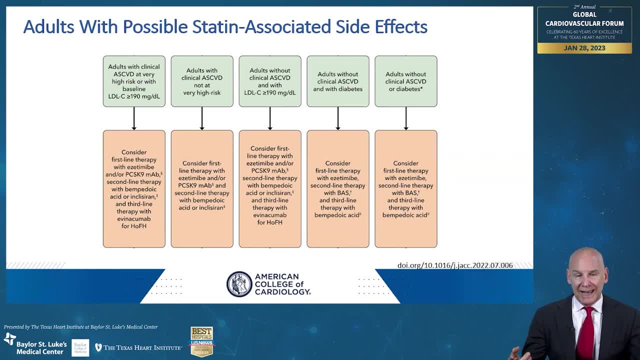 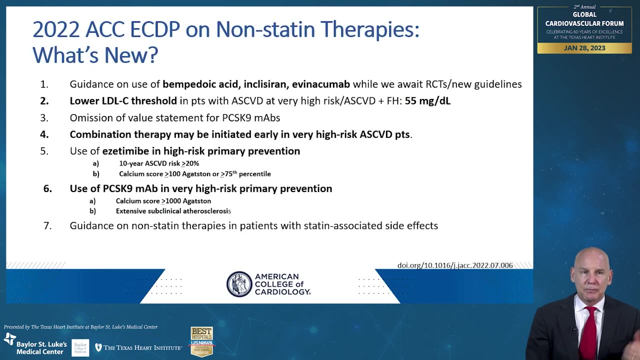 PCSK9 inhibitors. consideration of using bimpedoic acid and glycerin. It's just very important And we have a high-risk patient who is not able to tolerate statin. We have the tools now to be able to get the levels of LDL down All right. so summary Guidance on the new therapies: bimpedoic. 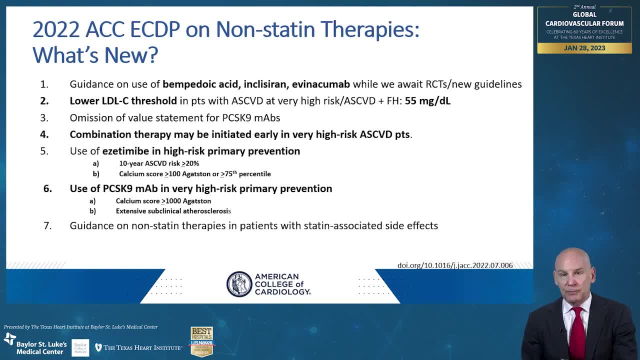 acid and glycerin. Evanacumab is really for homozygous FH- A lower LDL cholesterol threshold 55, now A combination therapy, starting it earlier, More of a role for ezetimibe and high-risk primary prevention combined with statins And also a role for PCSK monoclonals- high-risk primary prevention. 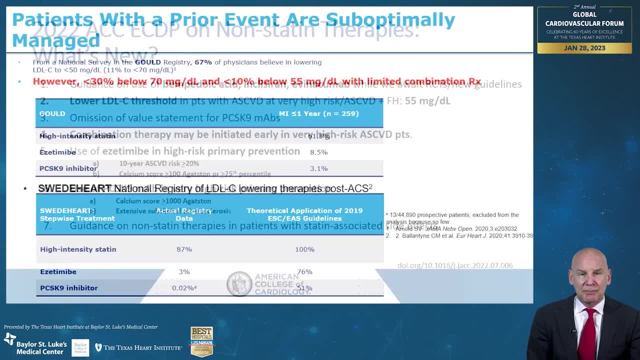 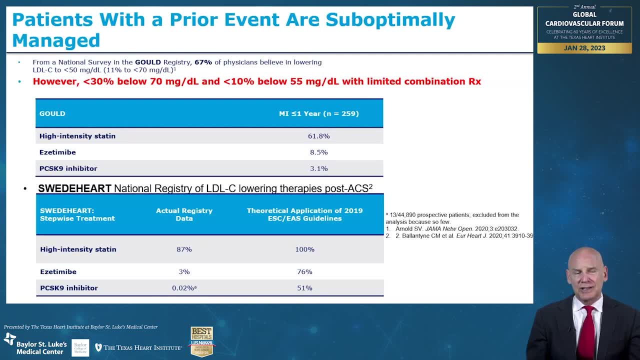 people with a very high calcium score. So what's happening in practice? Well, what's happening in practice is we don't see much combination therapy. This is data from the Gould Registry, which I was a part of, but we see the same in Europe, all over the world. There is very little combination therapy Now, in contrast. 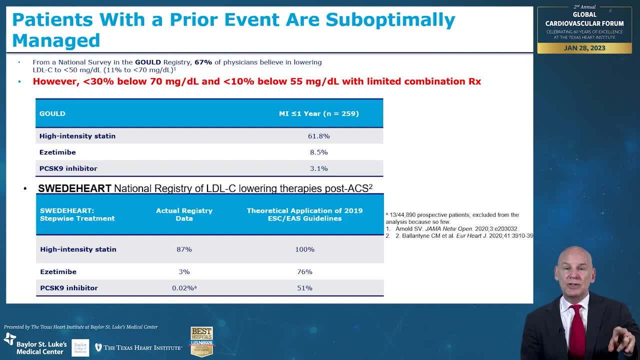 the people in the Gould Registry for hypertension, 70% were on combination therapy for hypertension. Why, Pragmatically, We know it works better, It's easier People, instead of pushing one drug up to the highest dose, we use combinations. Time to start doing that in lipids. 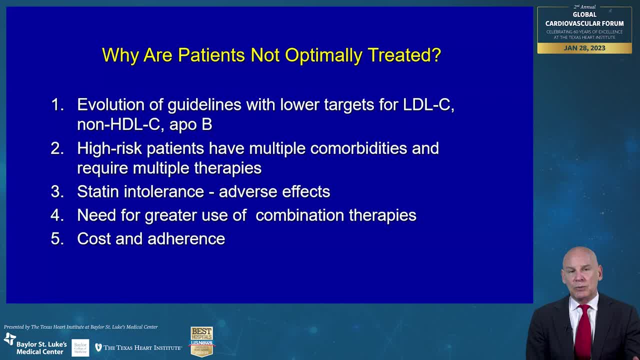 I think So. why are people not being well treated, to their targets? Well, the guidelines have lower levels. These people are on multiple therapies. Sometimes we have problems with people tolerating the highest dose of a high-intensity statin. I think we can use more combination therapy. 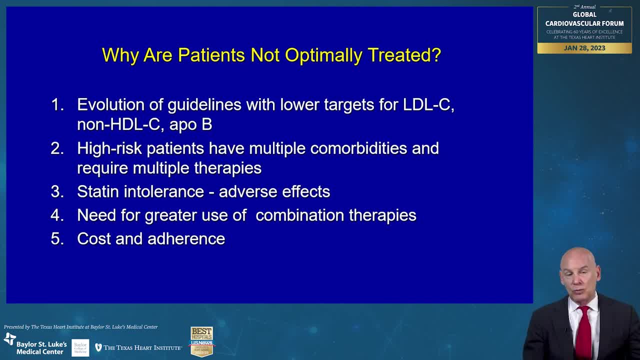 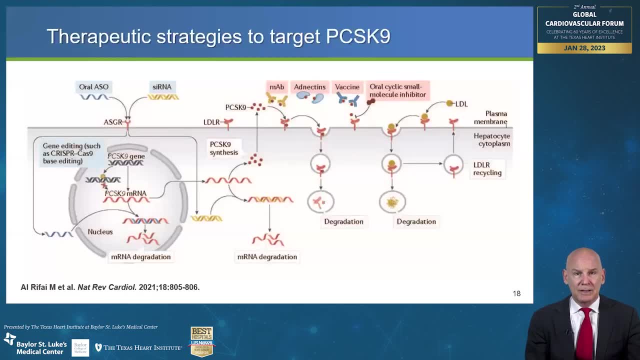 And then there's also the issue of talking to your patient. What about cost adherence? If we're going to use an injectable, are they willing to do that? Frequency of the drugs, et cetera. Now, what's going on in this field right now? PCSK9 has been a very exciting story, As mentioned. 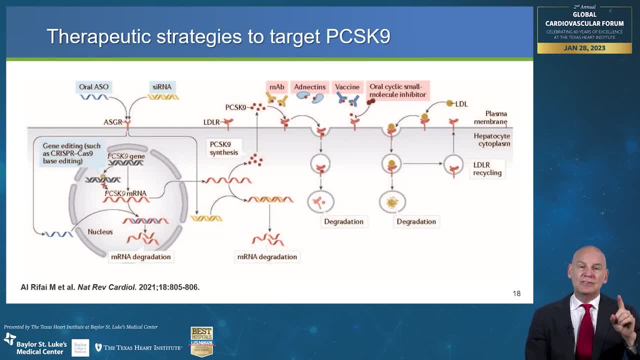 you know, we start off with the monoclonal antibodies. We have an S-IRNA that's in clostrin. You have a dose in three months and every six months. We're starting trials with CRISPR-Cas9, which would be once in a lifetime. Those have been started in Europe. 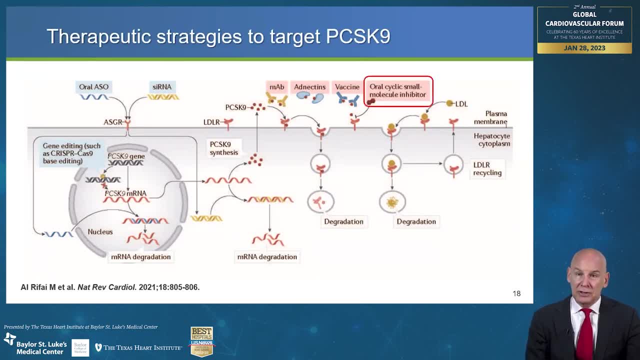 They'll be moving to the United States sometime soon. And also we now have data on an oral PCSK9 inhibitor And stay tuned. I'll be presenting this at a late-breaking trial at the ACC in March, but another exciting option that's moving forwards. In addition to LDL, there's also. 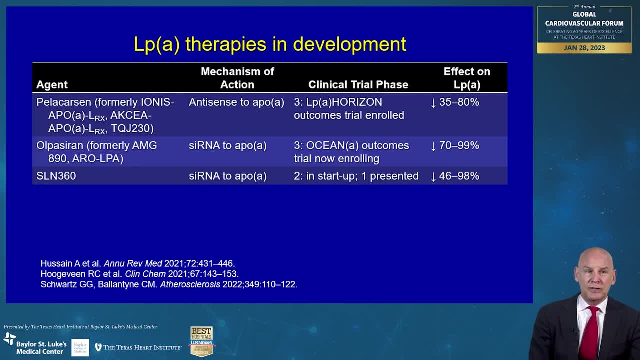 the issue of lipoprotein A, And there's a lot going on in this field. We've got an antisense oligonucleotide, a fully enrolled outcomes trial called HORIZON. We've got a small interfering RNA that's called the OCEAN study, And this would be used less frequently. S-IRNAs are longer. 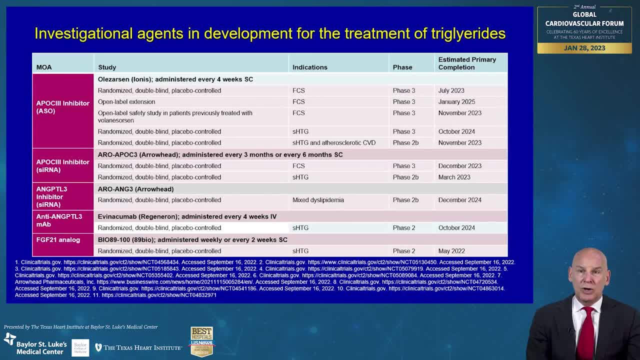 acting And there's a drug in the pipeline. What about triglycerides? A lot of things happening here also, And once again we see, is that with genetics you identify new targets. APOC3, we have antisense oligonucleotides, We've got small interfering RNA molecules. 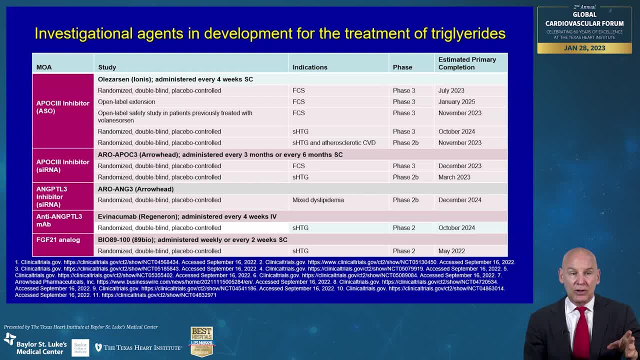 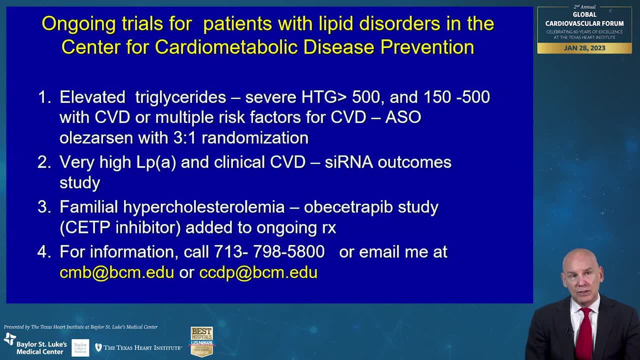 ANGPTL3, small interfering RNA program, for that also. And then FGF21 analog is another exciting drug in the pipeline. All right, So I went over quite a few things with it. We covered the ACC expert pathway. Remember we have a new lower threshold from that- more combination. 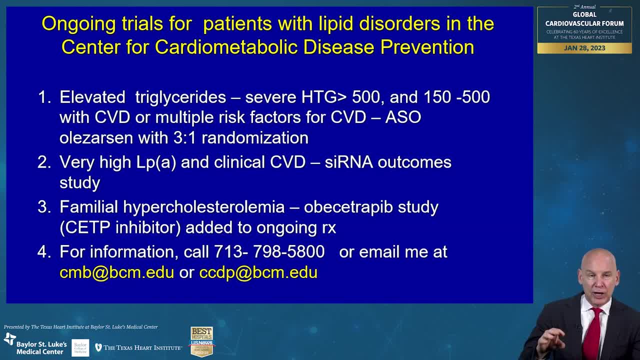 therapy. I talked about a lot of new therapies that are in the pipeline And let me just put a plug in right now. We are actively recruiting for people with high triglycerides. We talked about these therapies. There are therapies that are ongoing, new targets with these, like APOC3 and antisense. 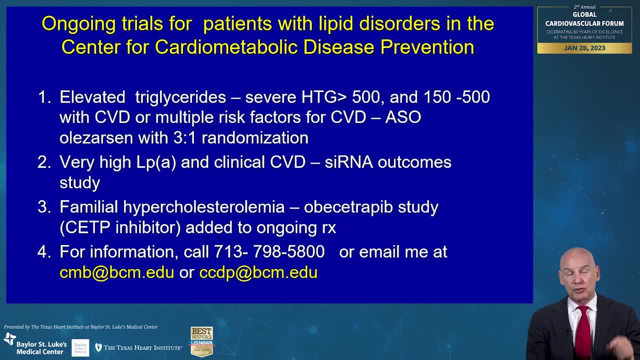 oligonucleotides high LPA. I hope it's something that you're screening in your practice. It's a very common: about one out of five people have a high level. Individuals with very high levels in clinical cardiovascular disease are being now randomized into a new outcomes. 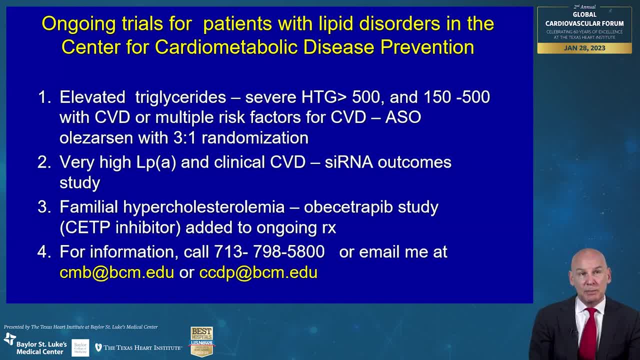 trial And there's a new therapy for familial hypercholesterolemia that's being tested. This goes back to a CTP inhibitor that recently been shown to reduce LDL. It's a pill 50% on top of statin therapy, So I hope that this has been informative. A lot going on in the field with it. 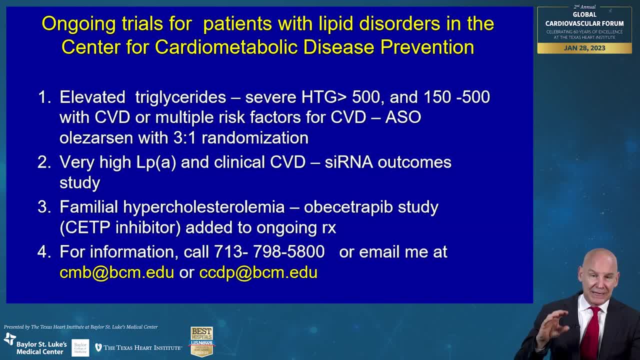 And the main thing is make sure that we do a better job implementing in practice. We want to do risk assessment for the very high risk patients. We want to be aggressive with those patients, Drive the LDL down to low levels. we've got the tools to do it now and we're not confined only to 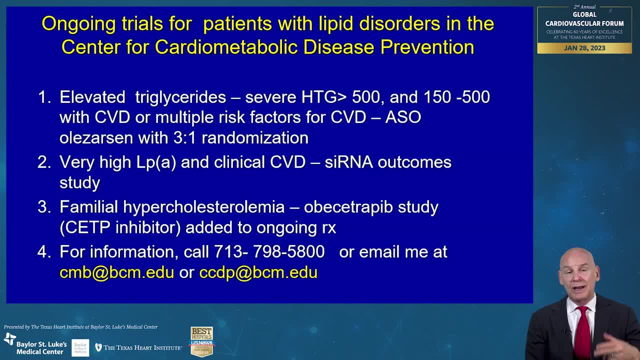 statin therapies, more going on in the fields with high LPA, high triglycerides, lots of very promising therapies. right now it's challenging: we don't have any to anything approved specifically for high LPA and we only have one therapy, icosapent ethyl, which is shown benefit in people with high triglycerides and 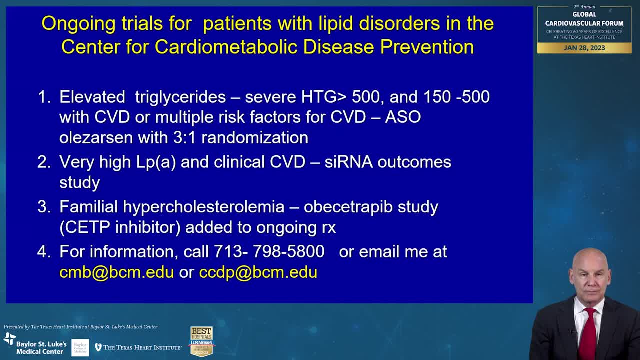 at the scrotum cardiovascular disease. thank you very much.